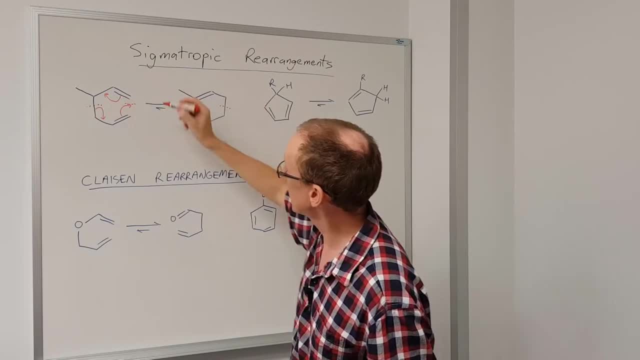 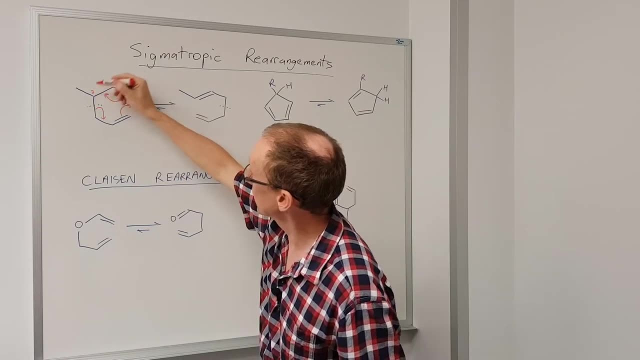 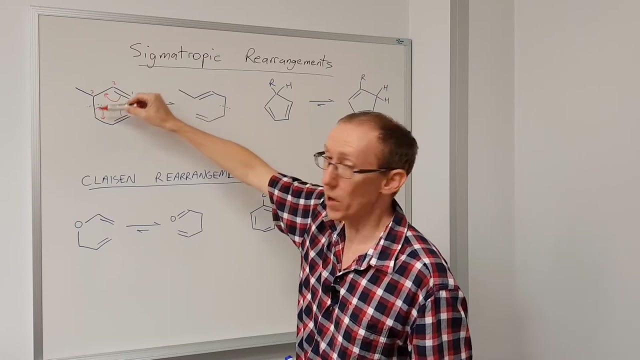 and it's being formed here. So we can see that there's sort of two halves to the molecule: The first half. if we number that like so we see that there's three atoms in that contiguous set of atoms that make up the ring at the transition state, And similarly there's three 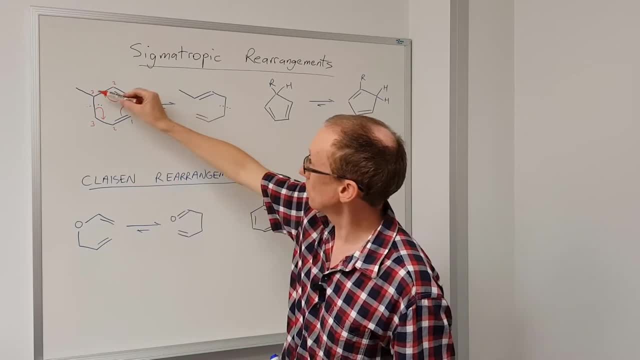 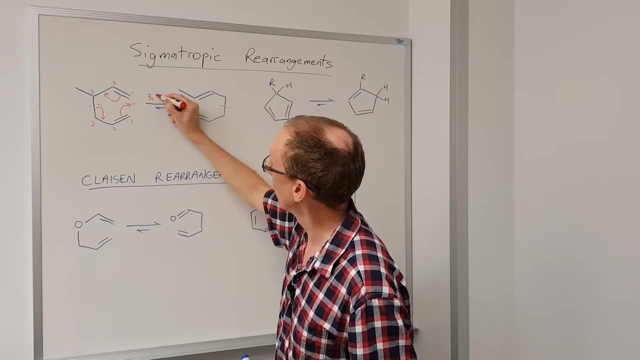 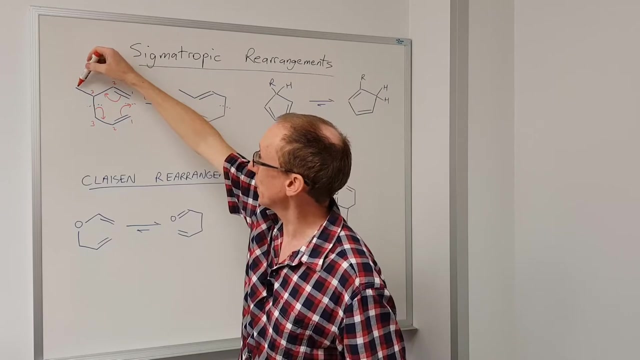 atoms on this side, And so there's three atoms on each side of the sigma bond that's being formed and the sigma bond that's broken, And so we call that a 3,3 sigmatropic rearrangement. Now it's important to note that this methyl group here doesn't get counted in the numbering. 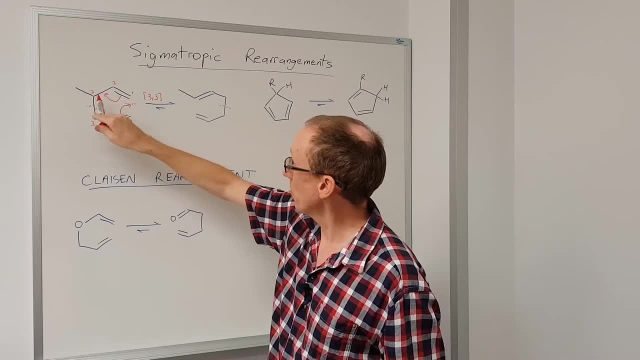 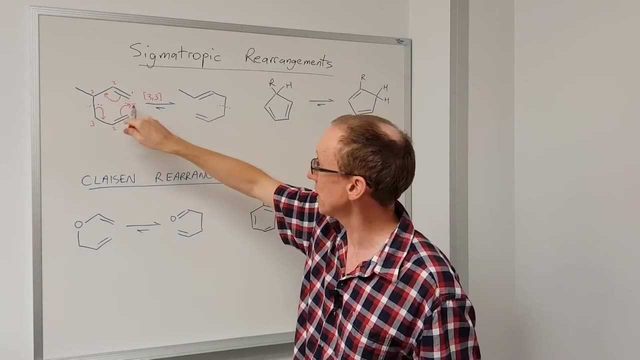 because, although it's attached to this group here, it's not part of the chain that's within the ring that forms the transition state, So it's not part of the contiguous set of atoms. So we can see that there's three atoms that are undergoing the reaction and involved. 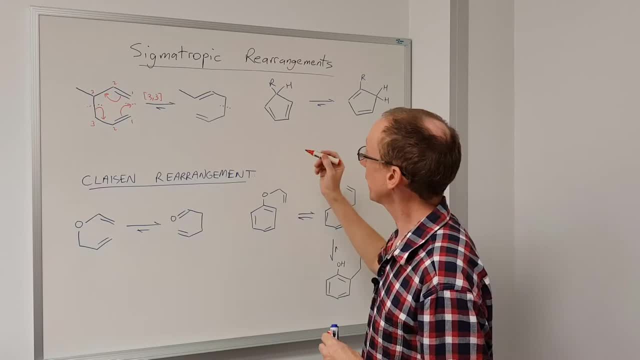 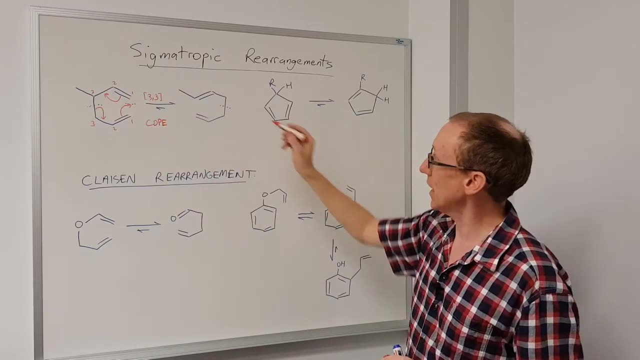 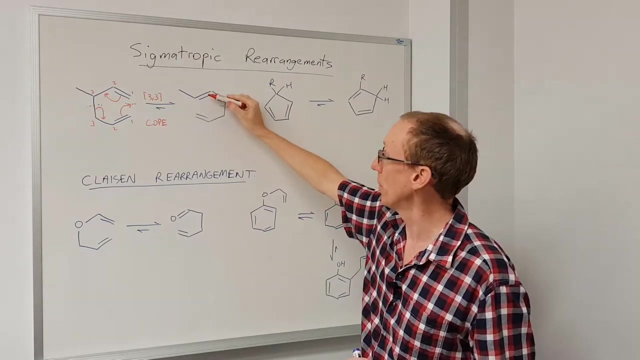 in the transition state of this reaction. Okay, so that particular reaction is called a Cope rearrangement. And how do we predict which side the equilibrium favors? Well, it favors this compound because it has more substituted double bond. So it's normally favorable for double bonds to have more alcohol and less. 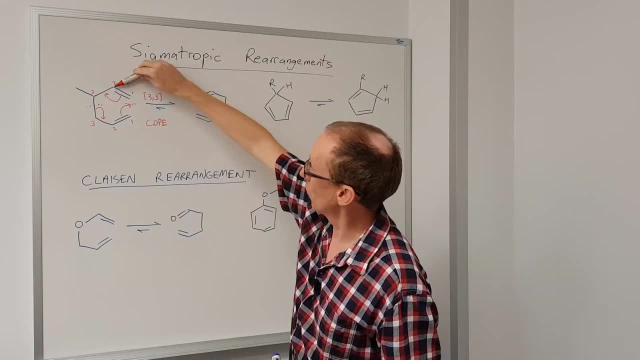 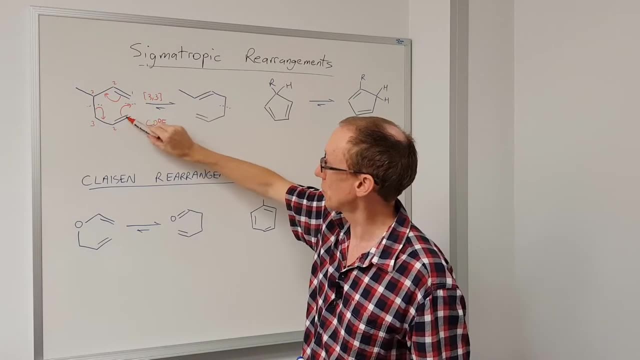 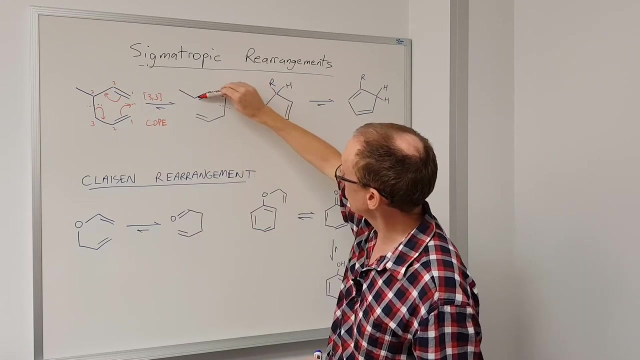 hydrogen substituents: A monosubstituted alkene here and a monosubstituted alkene here. So there's three hydrogens and one alcohol group, three hydrogens and one alcohol group, Whereas over here we have a disubstituted alkene and a monosubstituted alkene. So this molecule is more stable because 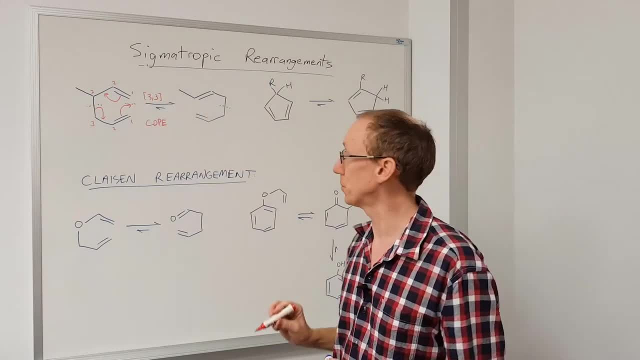 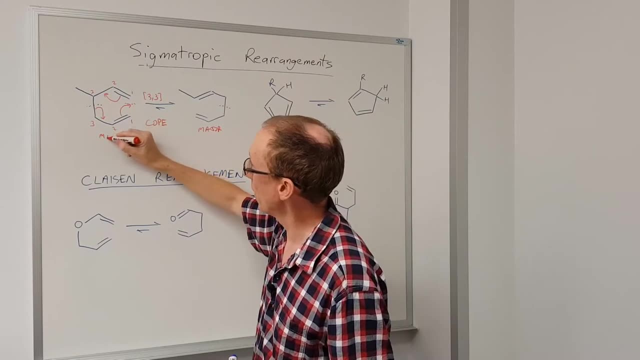 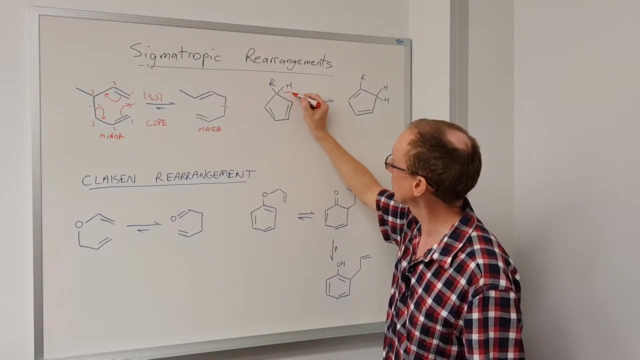 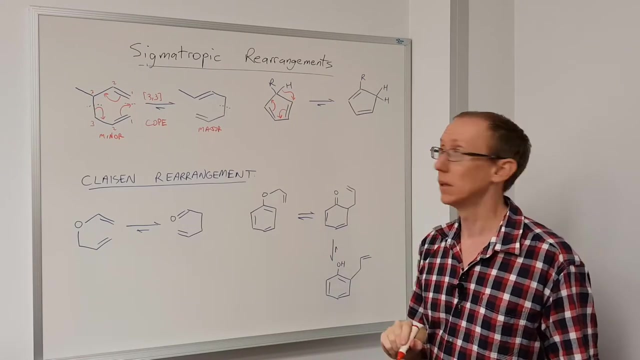 we have one alkene with extra substitution, And so this will be the major component of the equilibrium And this will be the minor. Okay, let's look at this example here. So, once again, curly arrows, we can show this hard drive migrating. move these pi electrons around the ring and we get to our product. 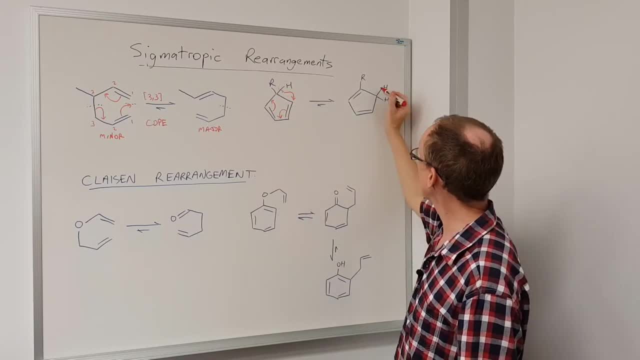 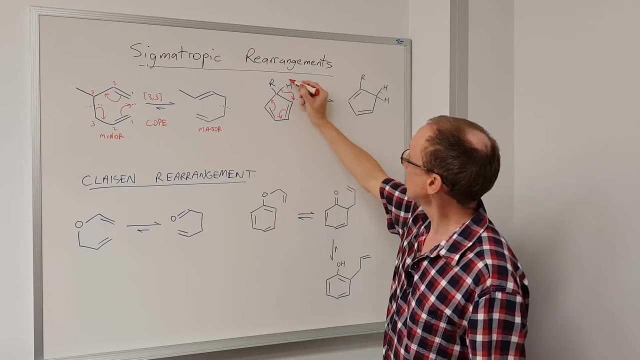 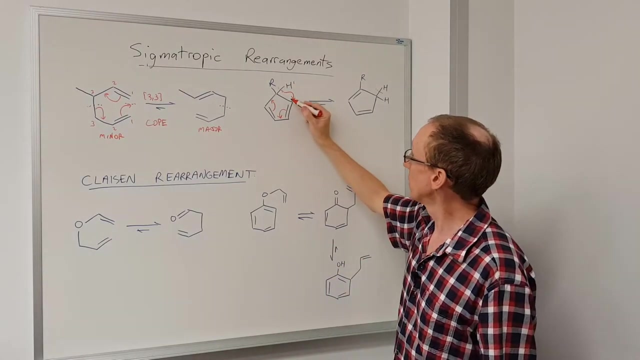 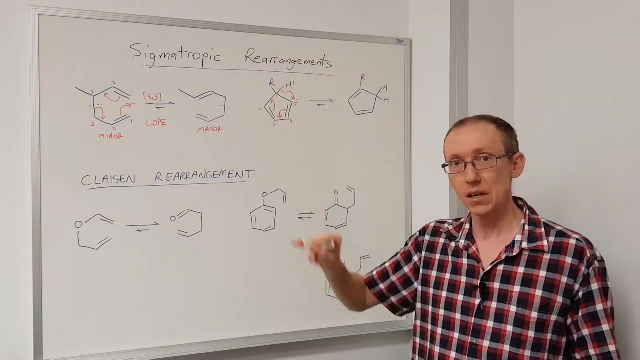 Once again, there's the sigma bond that's breaking, Here's the sigma bond that is forming, And so there it is, there that's forming. So on one side, the group that is migrating is only one atom in size, Whereas on the other side, we've got one, two, three, four, five contiguous atoms that. 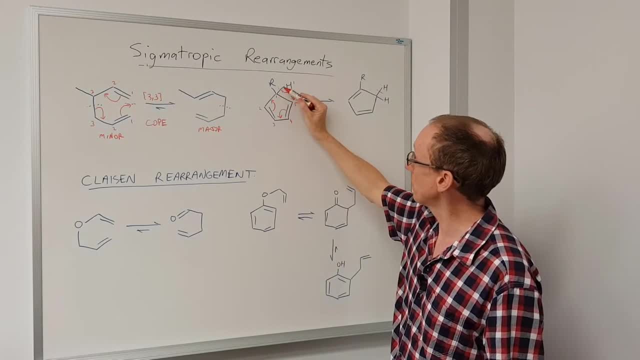 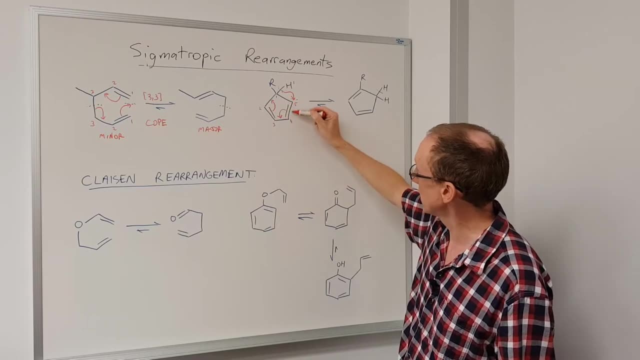 are forming up the chain that is involved in the sigma bond that's breaking and the sigma bond that's forming. If we had other substituents here, they would get counted. We just look at the atoms in that chain. that is part of the transition state. 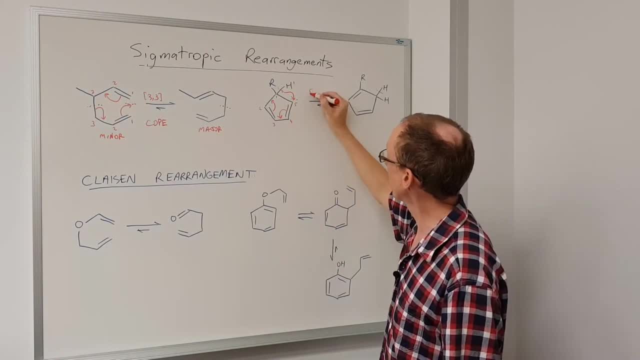 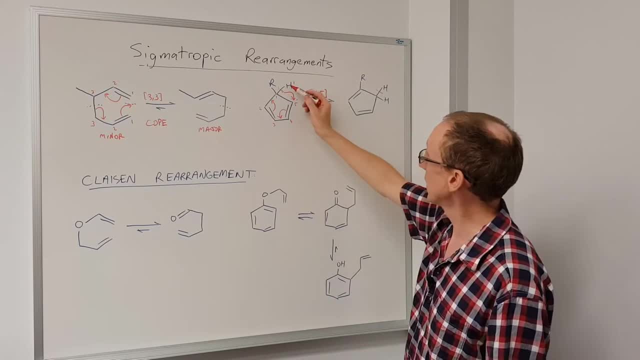 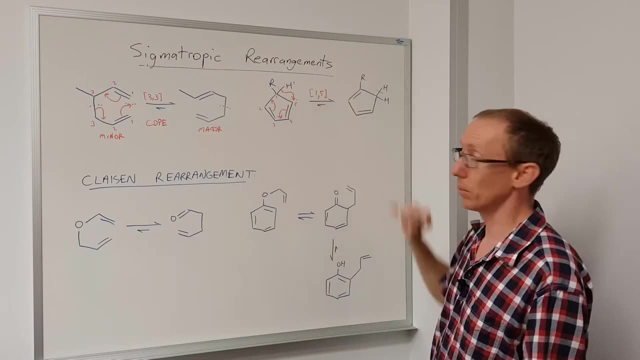 And it's a hybrid that's moving, So you could also call it a 1, 5 hydride shift. And it's a 1, 5 hydride shift. Now, where does the equilibrium lie for this compound and for this reaction? 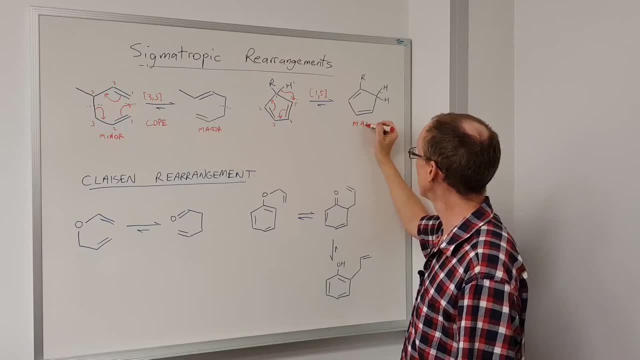 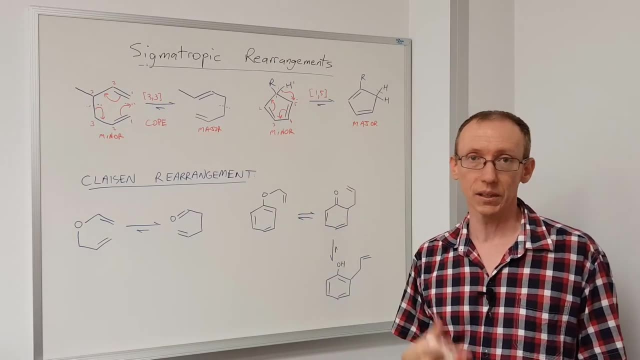 Once again it lies towards the right-hand side if we are assuming that the R group is some alkyl group like a methyl group and so on, Because here we've got a more highly substituted double bond than we have in the N group. 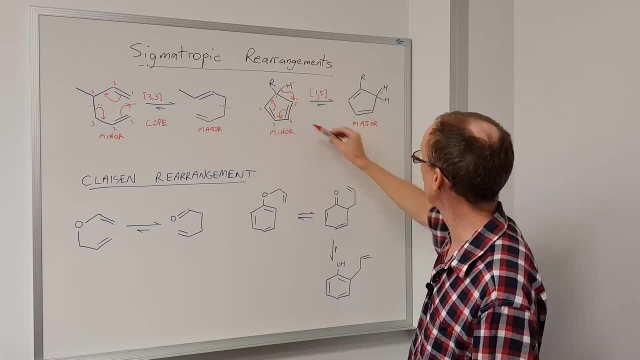 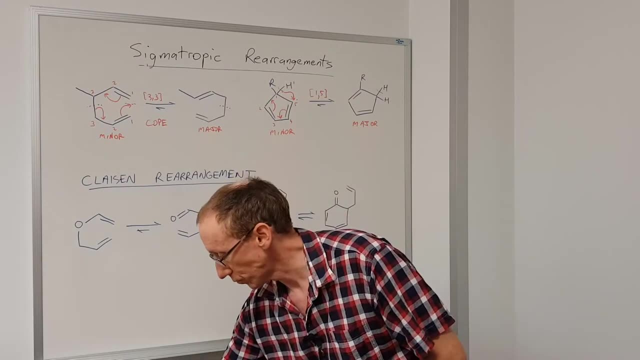 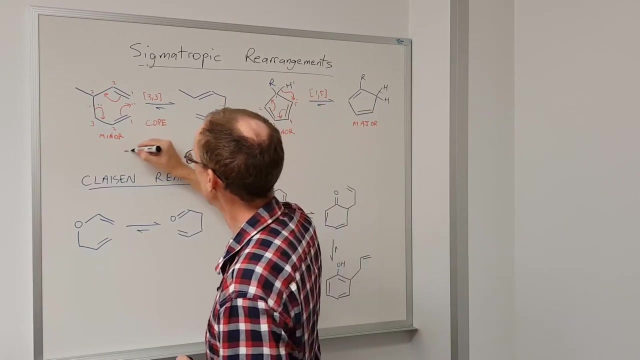 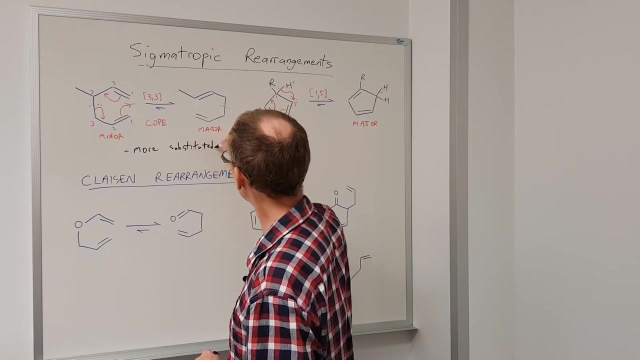 that we have in this molecule we've got two disubstituted, whereas here we've got a trisubstituted and a disubstituted. okay, so an overall key concept amongst these sorts of rearrangements is that the more substituted alkene 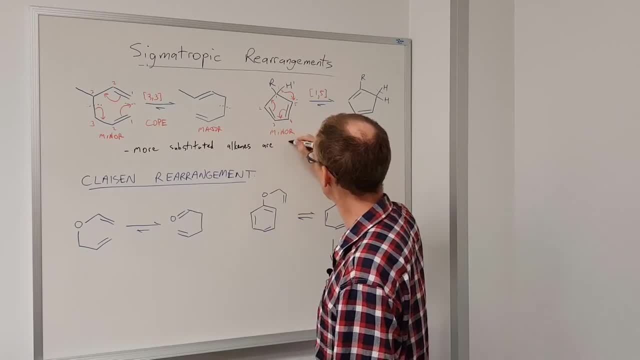 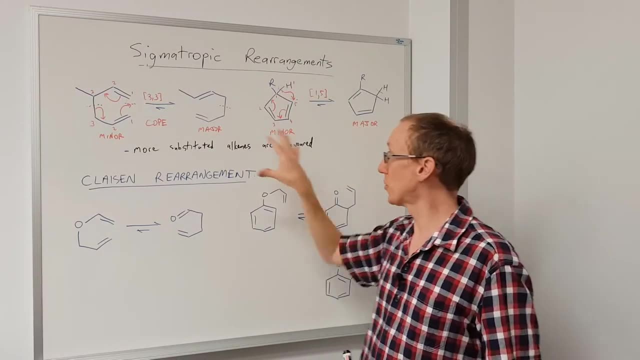 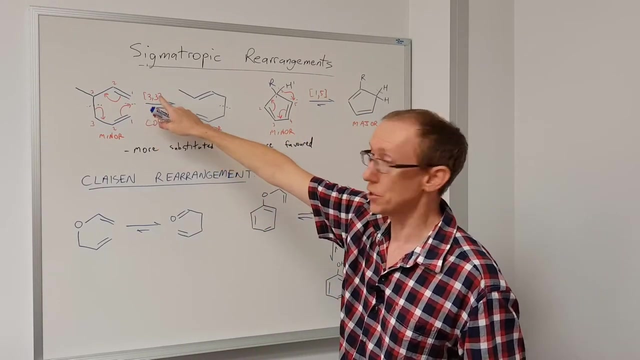 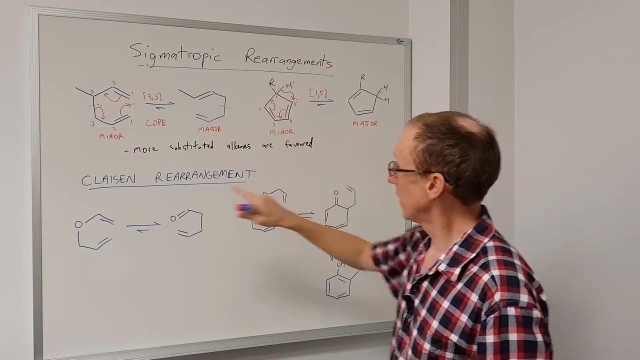 are favored, and so we could use that general rule to predict which side the equilibrium will be favored. okay, so that's the COPE rearrangement, which is a 3-3 sigmatropic rearrangement and 1-5 hydride shift, a very important type of 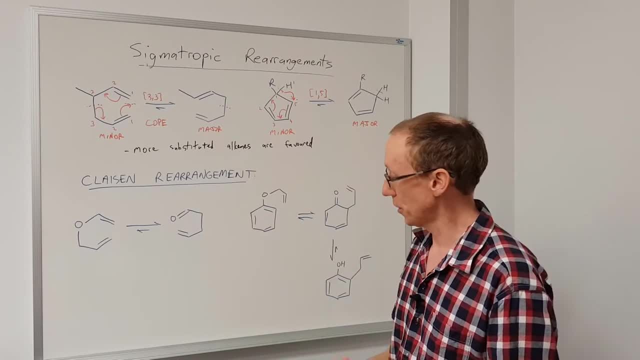 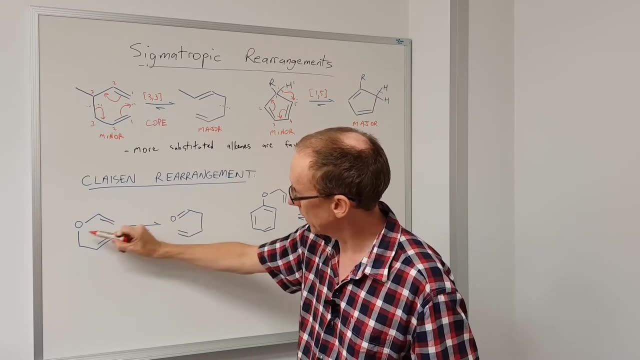 sigmatropic rearrangement is the Claisen rearrangement, so a 3-3. here's the simplest case. This involves a vinyl-allyl ether. So a vinyl group is where you have an alkene directly attached to something, and an allyl group is where we 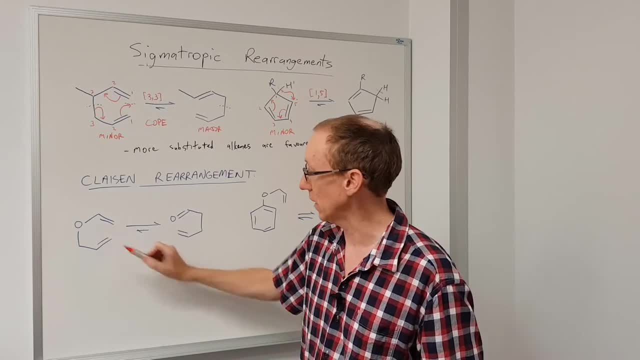 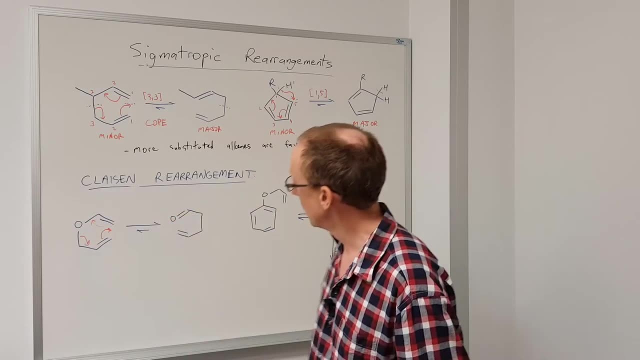 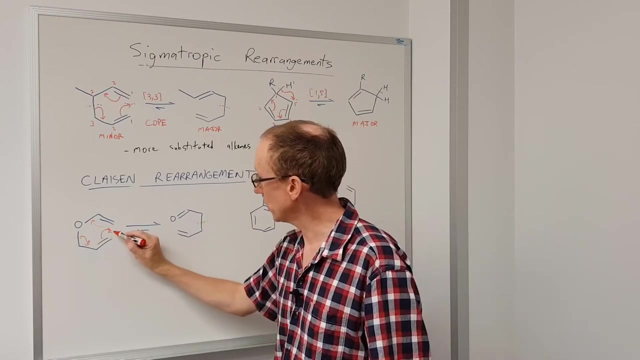 have a carbon, CH2, and then a double bond, so that's an allyl group, And the curly arrows can be drawn like this to show how the product forms: There's the bond that's breaking, There's the bond that's formed, So there's where it's going to form there. 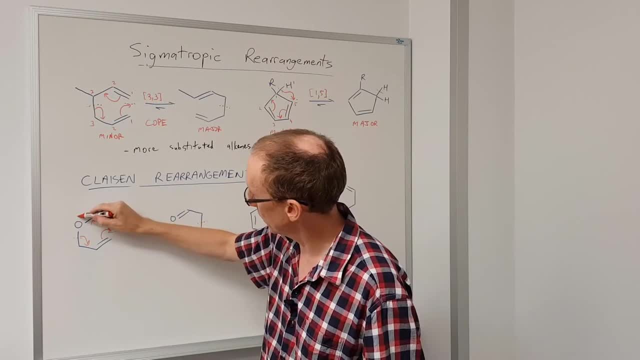 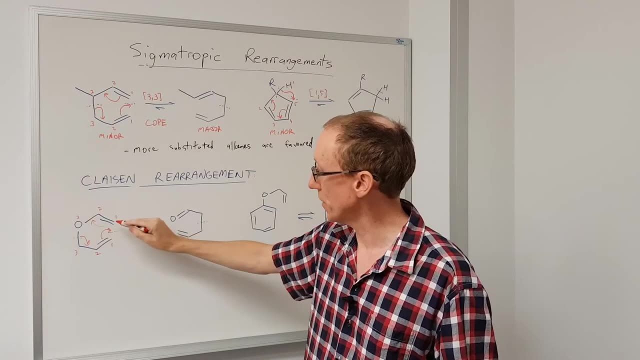 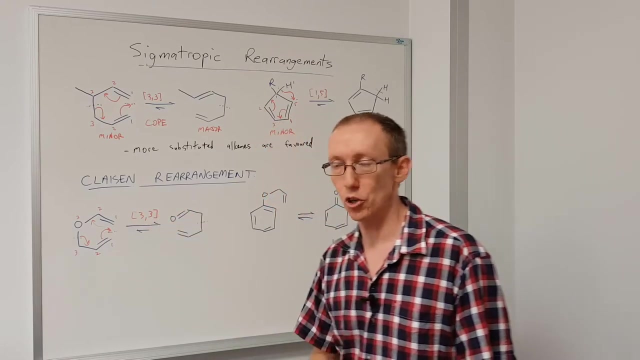 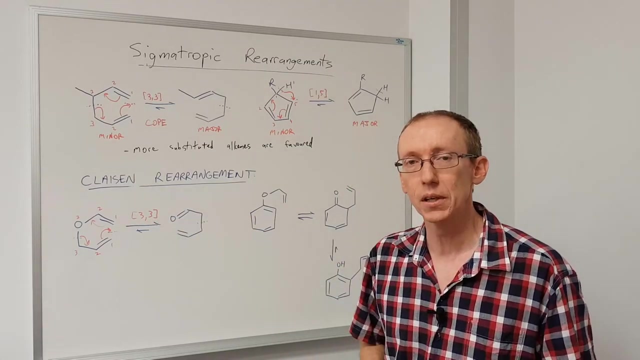 So once again we number one side versus the other. There's three atoms on one half of this transition state and three atoms on the other. so this is also a 3,3-sigmatropic rearrangement. This one lies over towards the right-hand side because carbonyl groups are particularly 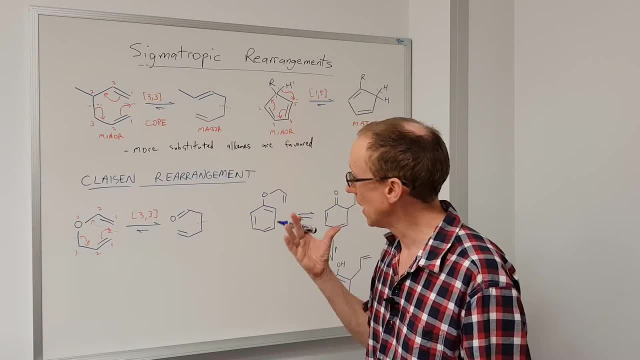 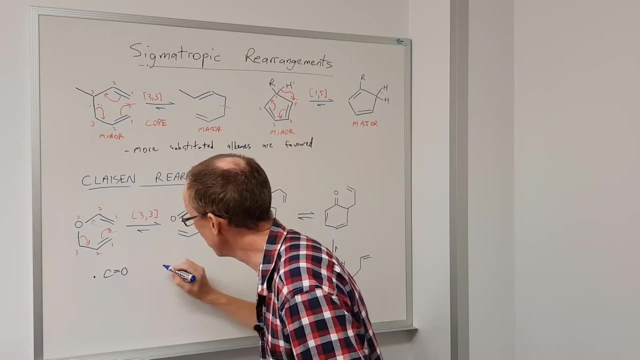 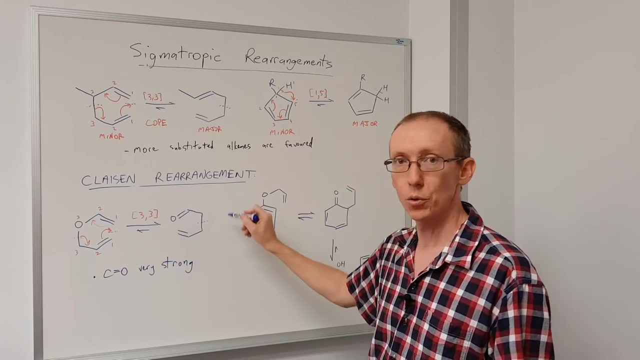 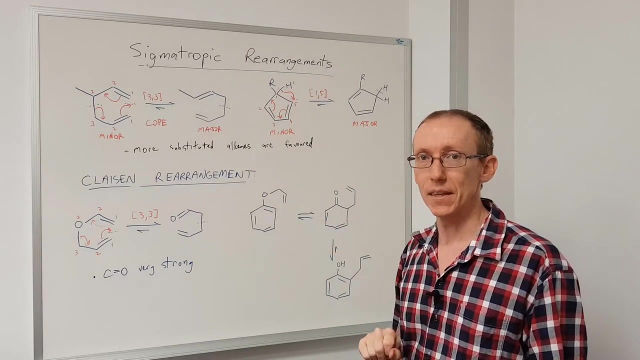 strong functional groups, so particularly energetically favorable. So CO double bonds are particularly strong, So CO double bonds are very strong And so therefore this lies over towards the right-hand side where we have that carbonyl group. A particular example of Klyzun rearrangement that is really important is the rearrangement of phenyl-allyl ethers. 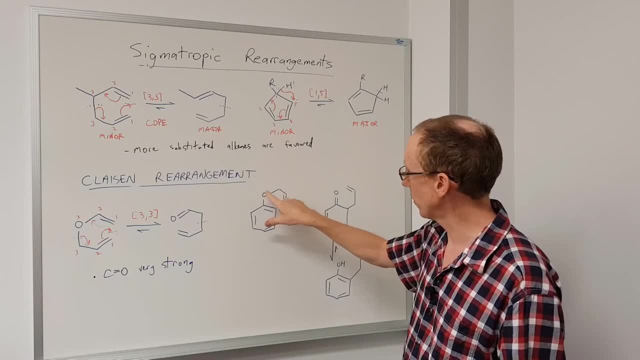 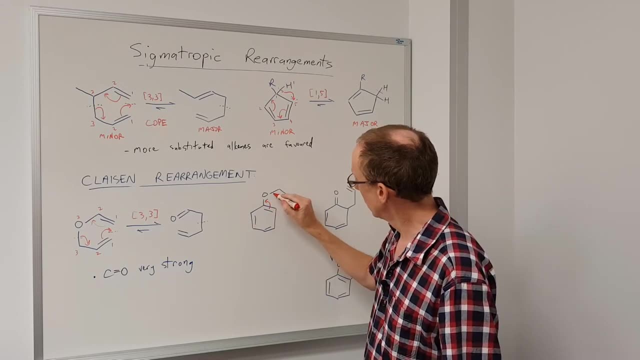 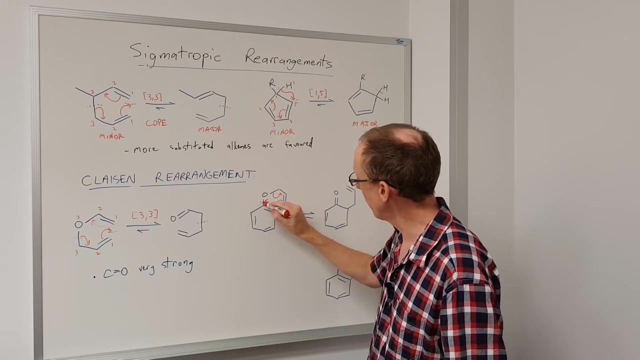 So this is where we have a benzene ring connected to an allyl group through an oxygen atom. So this can undergo exactly the same sort of mechanism: Electrons moving around in a circle like this. We've got the new bond being formed here, the old bond being broken there. 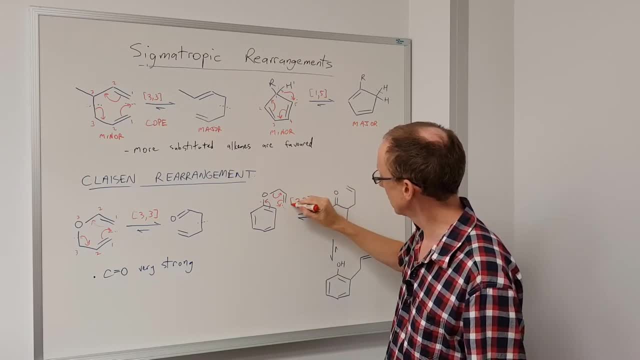 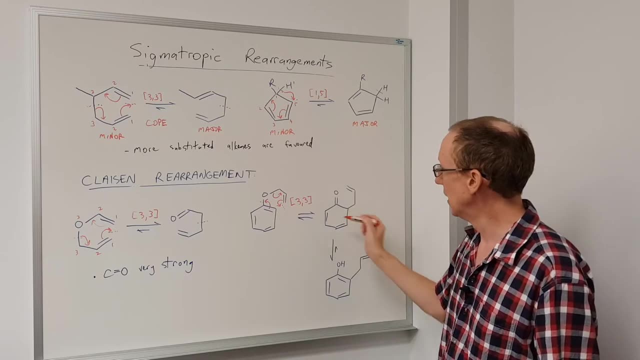 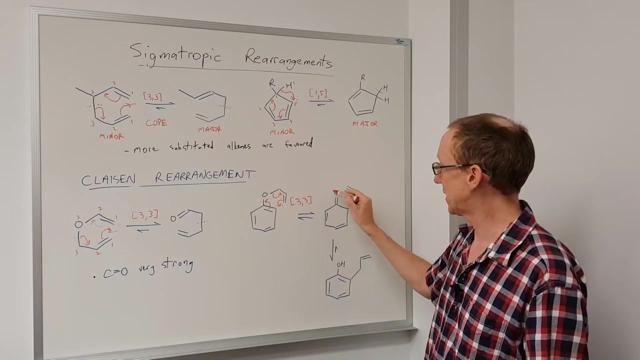 So this is also a 3,3-sigmatropic rearrangement. However, the product has this ketone in a very special arrangement, So this is actually you could think of this as being not a good thing, because you're losing aromaticity of this benzene ring, but it's somewhat made up for by the fact that carbonyl 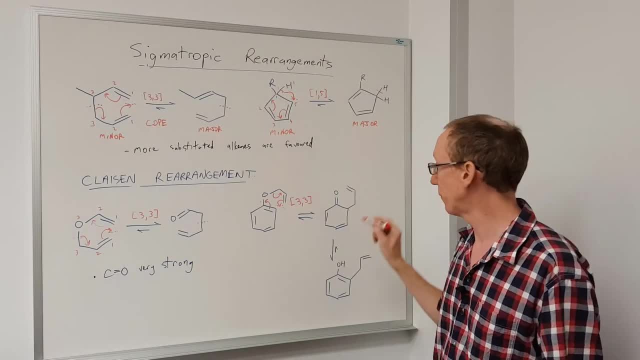 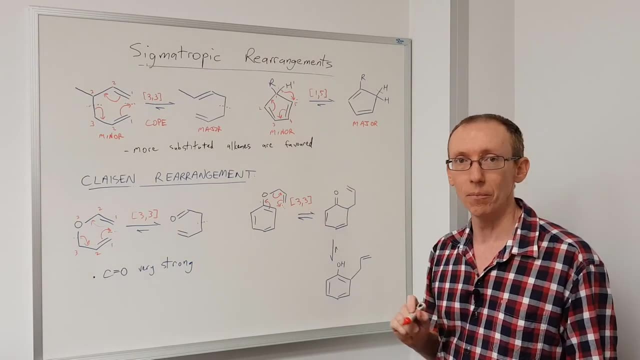 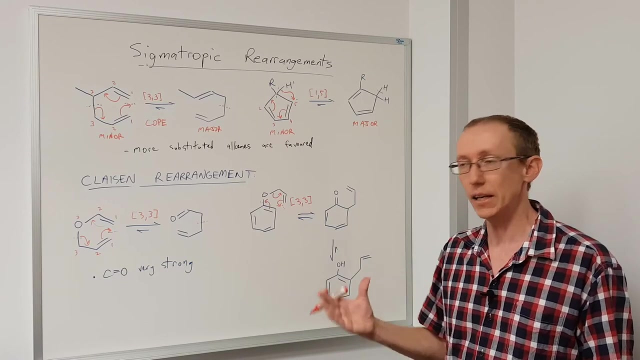 groups are particularly strong. The Klyzun rearrangement for these sorts of compounds doesn't stop there, because we know that ketones are, they can tautomerize to an enol form And there's always going to be that possibility of enol-keto-tautomerism. So that's the keto. 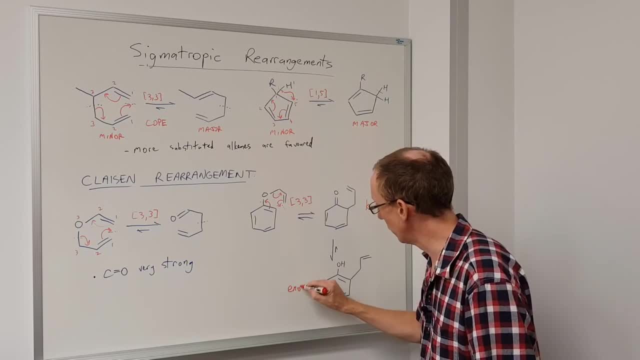 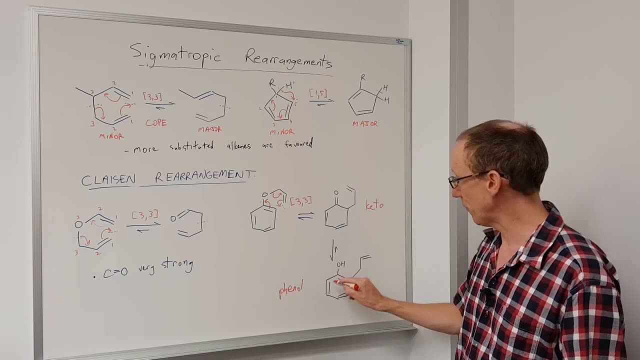 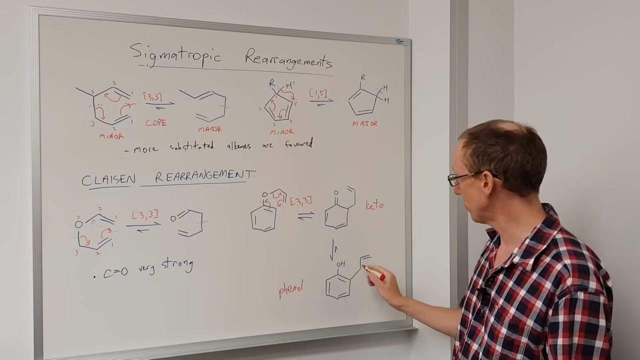 form. This is an enol form. However, it's a very special enol form. It's a phenol, And phenols benefit from aromaticity, and so this is going to be the major product by far at equilibrium between these two. So, overall, the Klyzun rearrangement of a phenyl-allyl ether goes. 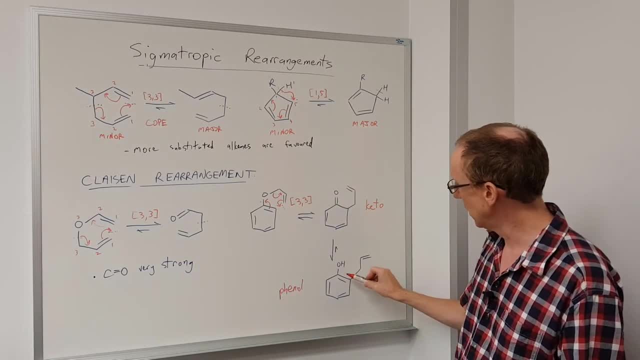 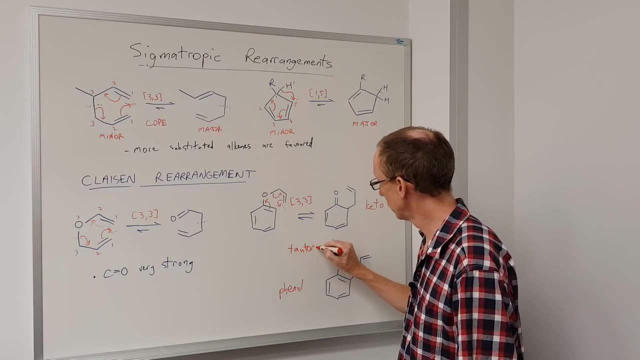 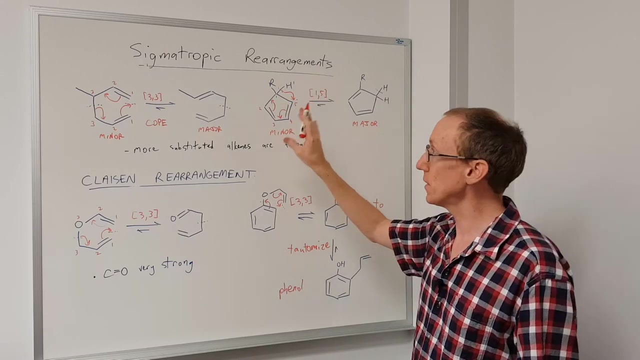 to give this initially, but you don't see that because it tautomerizes. to give the ortho-allyl-phenol Tautomerizers. Okay. so that's sigmotropic rearrangements, How to number them and a couple of most important. 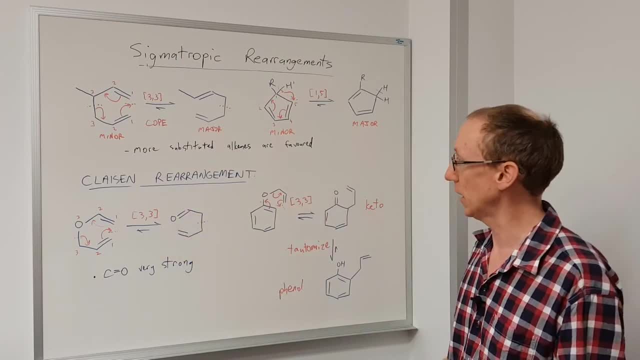 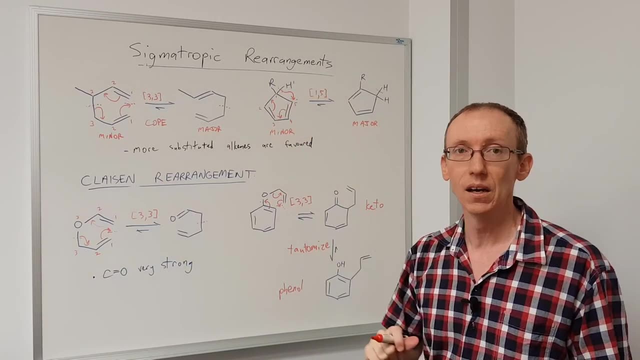 variants: The Koch rearrangement, 3,3-sigmatropic rearrangement including oxygen, which is called the Klyzun rearrangement, and 1,5-hydro shifts, which are particularly important in cyclopentadienes. you. 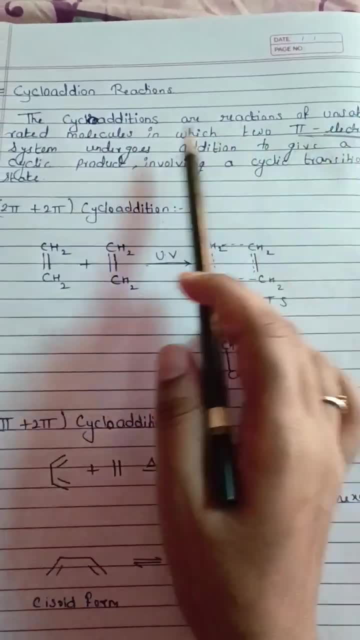 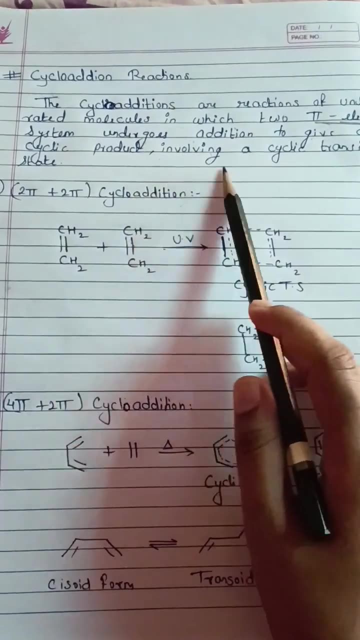 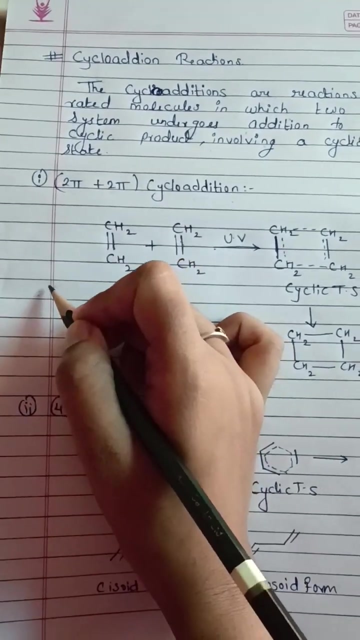 cycloaddition reaction. the cycloaddition are a reaction of unsaturated molecules in which 2 pi electron system undergo addition to give a cyclic product, cyclic product involving a cyclic transition state. you can see here the example: 2 pi, 2 pi cycloaddition. why we will call it is 2 pi, 2 pi electron: 2 pi, 2 pi. 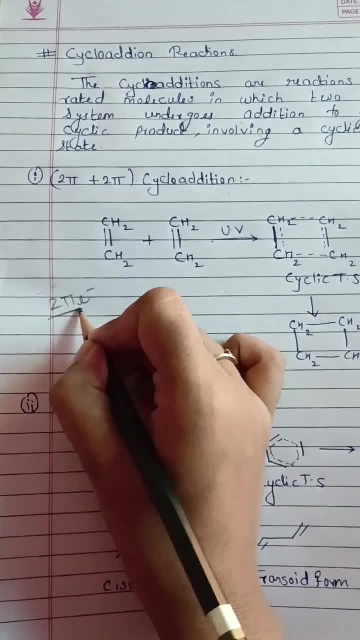 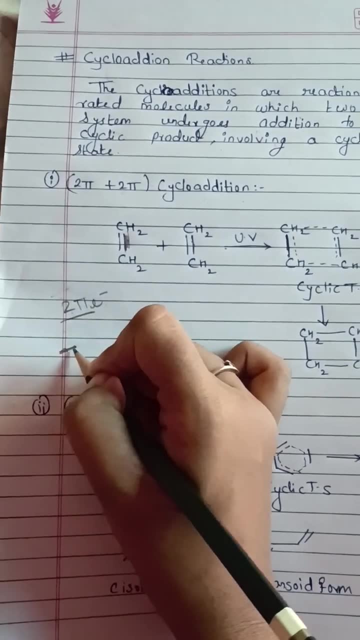 cycloaddition, because here the 2 pi electrons involved. okay, what is mean by 2 pi electrons? 1 pi bond: okay, this 1 pi bond contains 2 pi electrons. you know that how many electrons are in a bond? 2 electrons are there, okay. 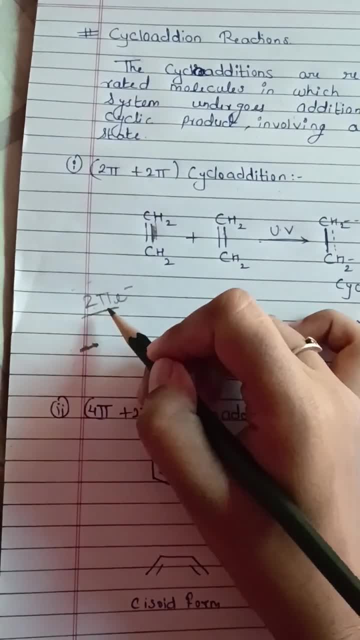 how many electrons are there? in one bond there are 2 electrons, so these two electrons are called 2 pi electrons in pi bond when 2 pi electrons are involved. now, in both of them 2 pi electrons are involved, so we call it as 2 pi- 2 pi cycloaddition. 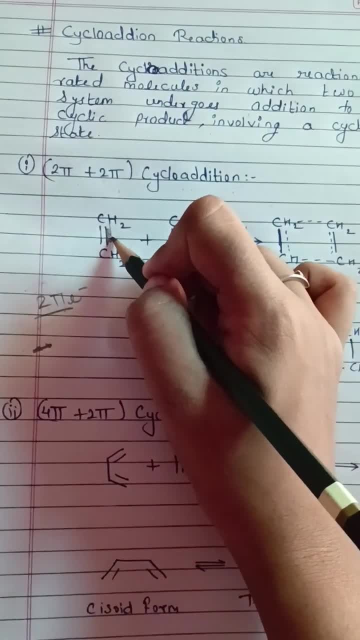 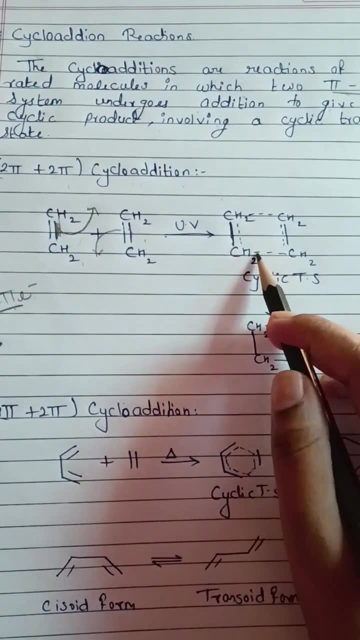 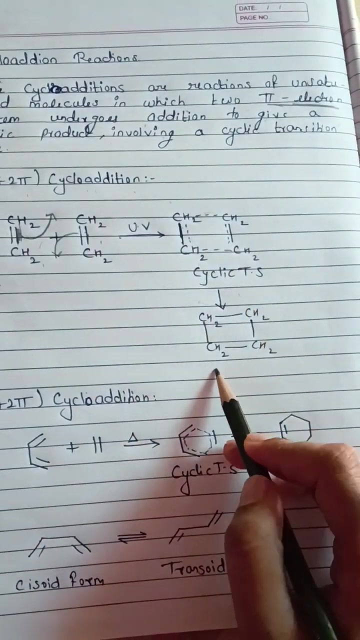 after this, what happens? this bond shift here, okay, and this bond shift is here. then what? here the broken bond form, or here the bond break. therefore, here the broken bond shows. now, this is a cyclic transition. state it and this is a final.